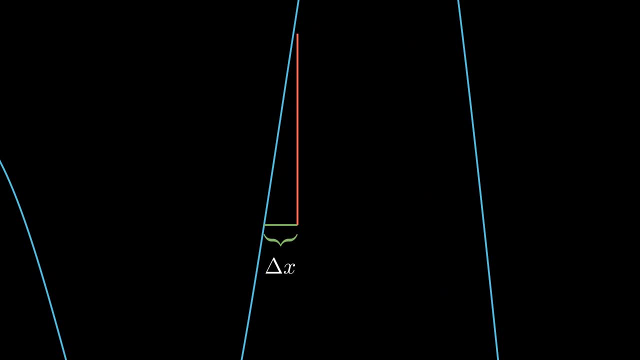 direction, which I'll call delta x. Again, this is a finite number. Let's call the resulting change in the function delta y. I'm going to call the hypotenuse of this triangle delta s. Take a moment to make sure you get everything. 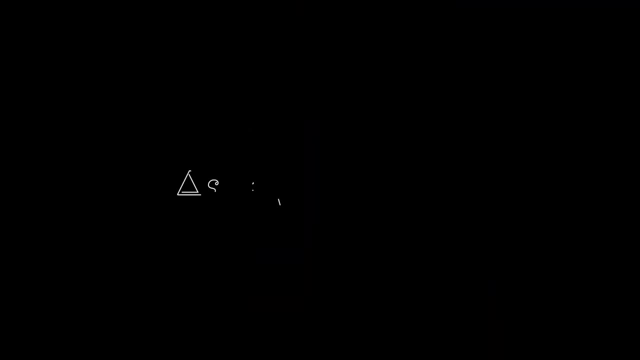 before I move on Now, delta s is the square root of delta x squared, plus delta y squared. Essentially, to calculate the arc length, we need to sum up all these hypotenuses. So let's do that. Now that we have a sum, we want to make our changes as small as possible. 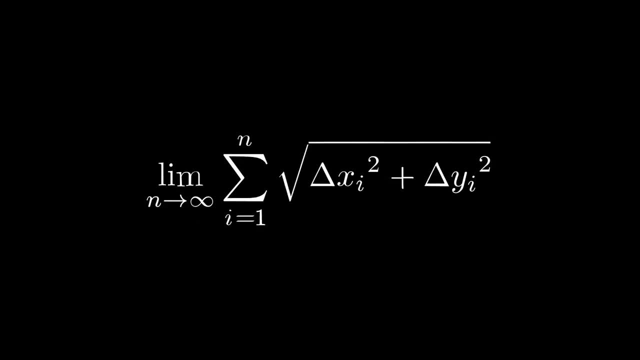 So let's do that. as n approaches infinity, This is the resulting sum. We can multiply and divide by delta t to get this sum. This is essentially an integral, which we can look like this: Now, this integral is commonly abbreviated as the integral from a to b, ds. 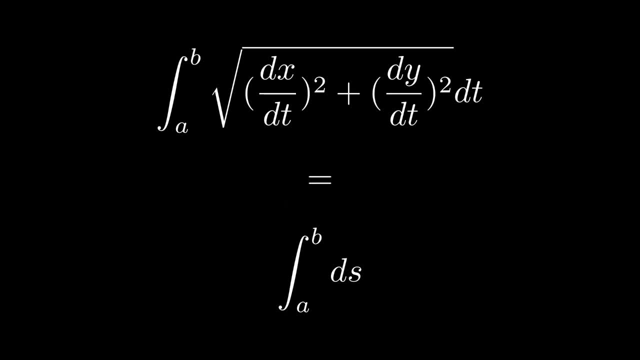 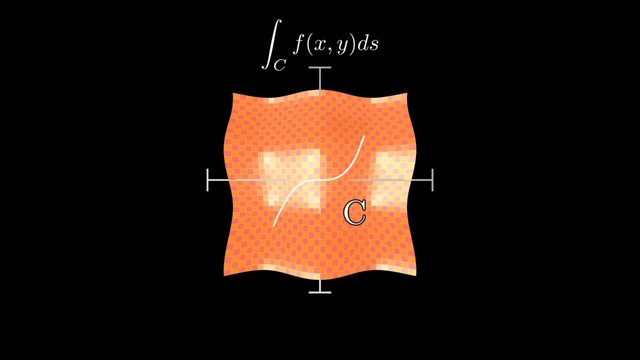 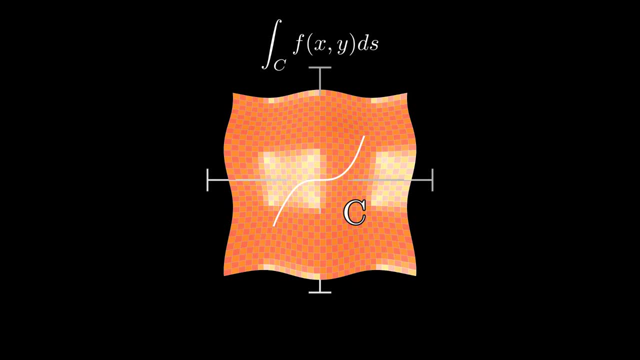 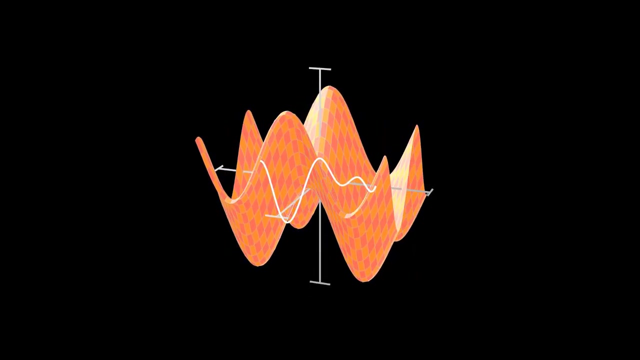 we get this line времени in today's original equation, it will be outside the graph. CCPAM has a convenient filling for unleashing these inequalities and limits. This is defined as a 2D parametric equation and we have f, which is a 3D surface. The brightest spots represent bumps, So let's. visualize this by rotating. This ends up laying our curve c on top of a 3D surface. The line integral is defined as summing up all the z values which c touches. Let's see what this means visual. we can project this orientation of f onto a 2d plane. and now, similarly, I can left and right this. 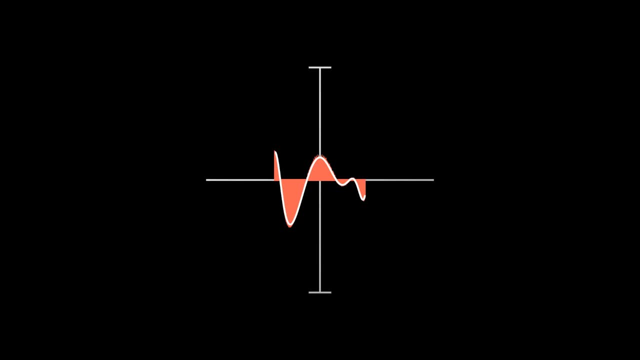 simply, it's a definite integral. Here we are summing up all the z values of f, of x, comma, y, for all values in c. In notation form it looks like this: Notice how we plug in the parametric equation into f and how ds expanded as we are going. 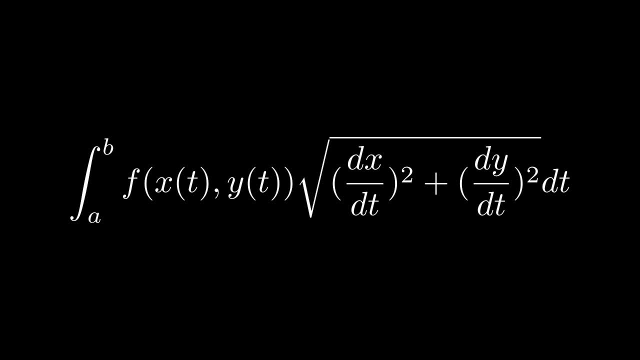 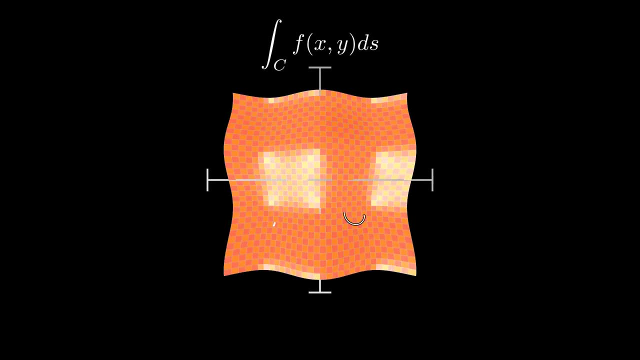 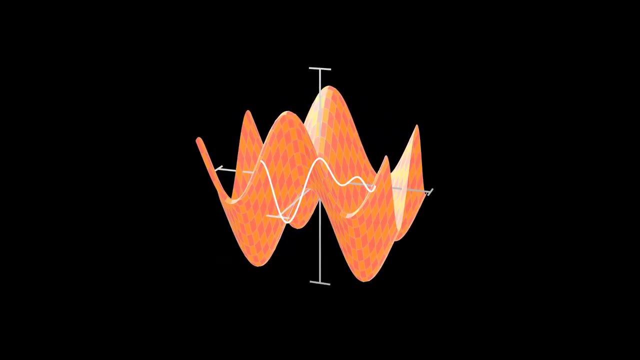 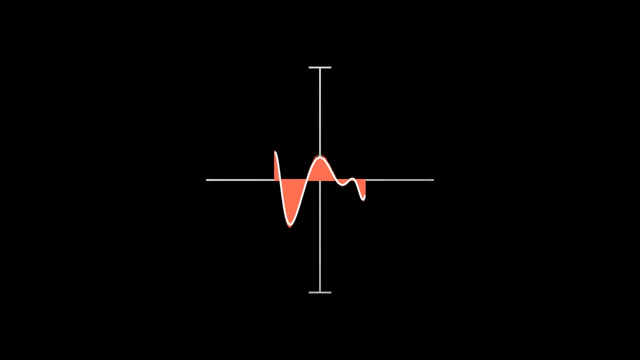 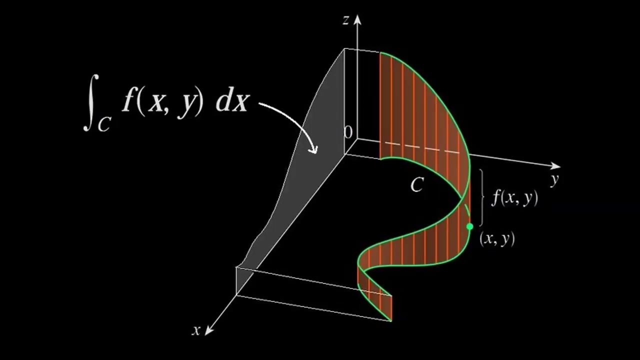 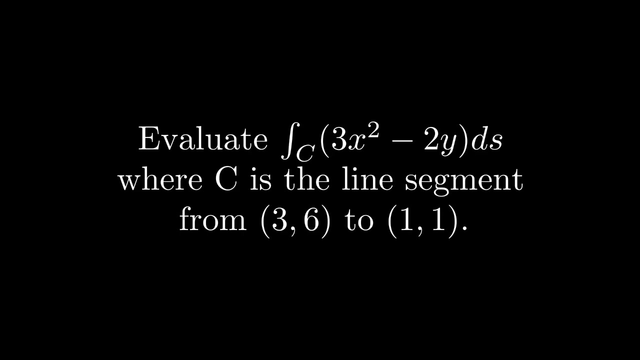 along a curve. I'm gonna play the animation once more for you to see again. Hopefully this picture also helps Now. I know a lot of people come here for help and also because they are interested in this topic, So I just wanna quickly go over a textbook. 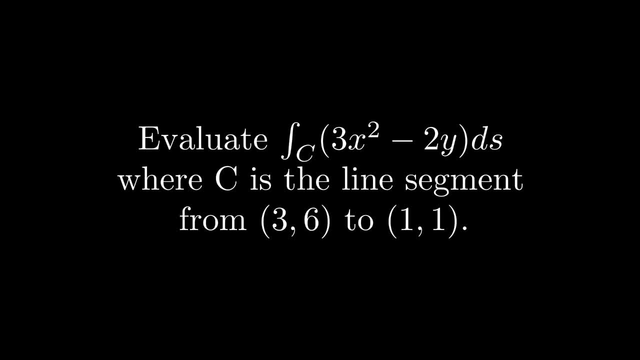 style problem quickly. So here's the problem. Evaluate the line integral of 3x squared minus 2 y ds, where c is the line segment from 3 comma 6 to negative 1.. So here's the problem. Evaluate the line integral of 3x squared minus 2 y ds, where c is the line segment from 3 comma 6 to negative 1.. 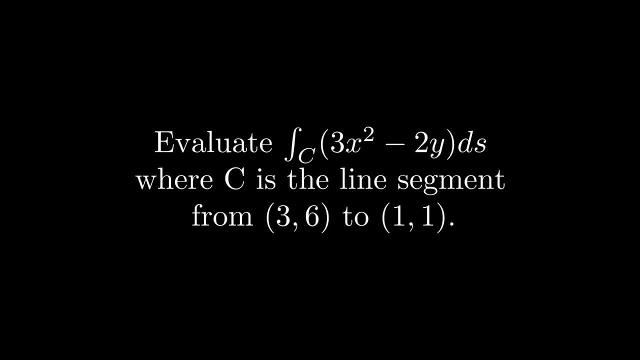 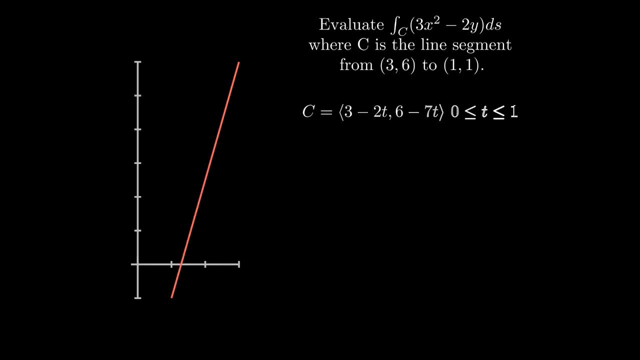 First I'm gonna graph c so we can get an idea of how it looks like. Next, let's parameterize the curve. It ends up being this: from t is equal to 0 to 1.. Now let's find dx by dt and dy by dt. Using our definition of ds, let's find ds. 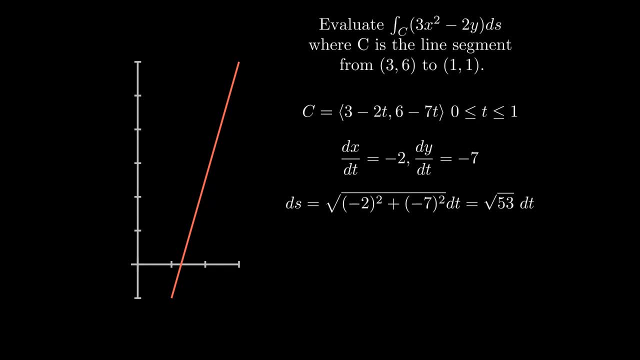 It happens to be the square root of 53 in this case. Using what we derived earlier, we can calculate this integral. Feel free to go back and recall this derivation Now. evaluating this, we get 8 times the square root of 53.. 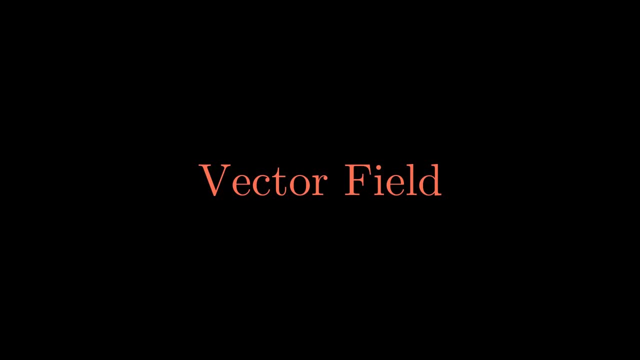 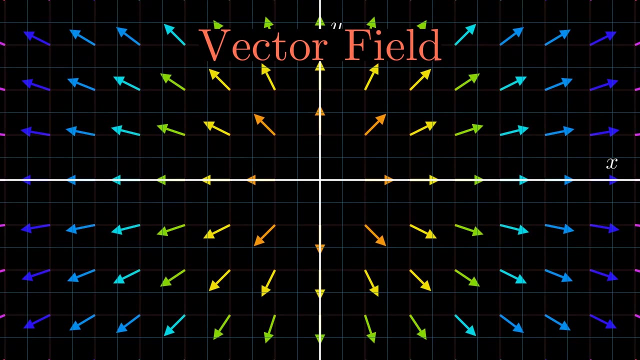 Now let's talk about vector fields. A vector field associates every point in space with a vector, like this- I'm going to use color because the lines get too long. So this vector field is the function of the vector field. This vector field is the function of the vector field. 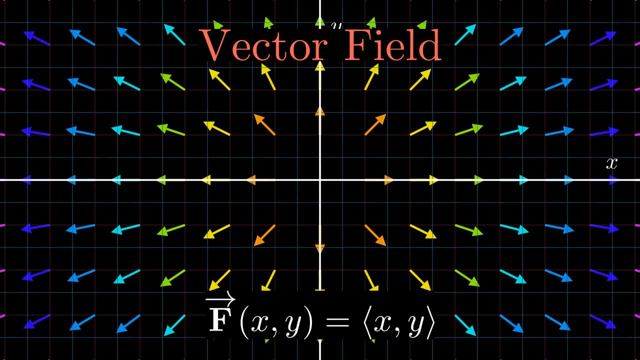 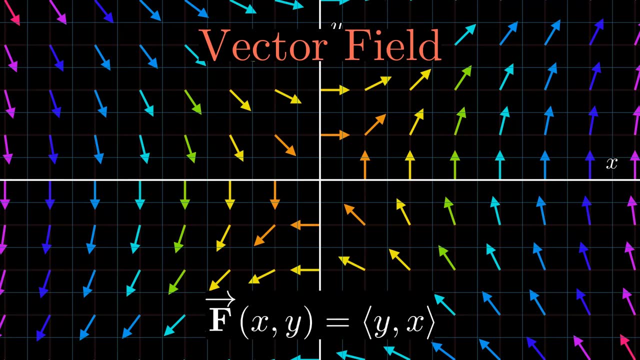 This vector field is the function. f is equal to x comma y. There are a lot of other cool looking vector fields like this one or this one. Vector fields are used to describe a lot of things like fluid flow, electric fields, magnetic fields, gravitational fields, etc. If you want to play around with vector fields, I've 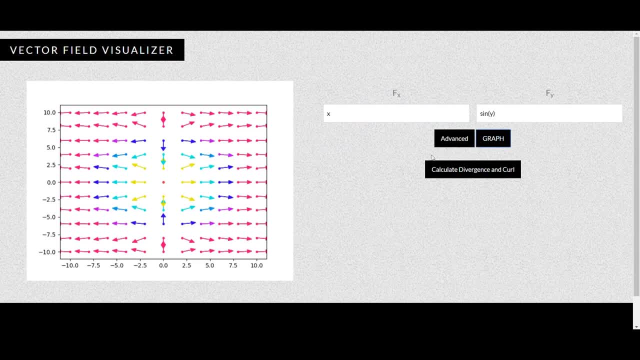 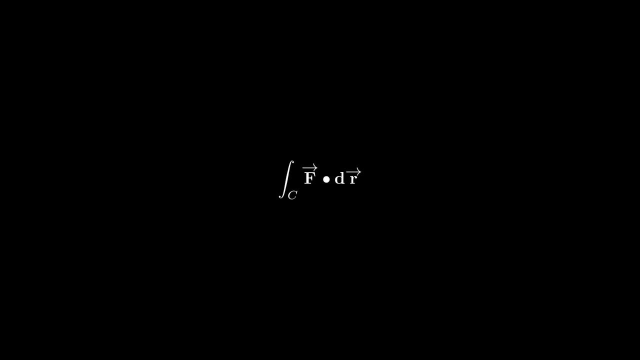 left a link to a website I created which can visualize vector fields and also calculate divergence and curl. I'll talk about divergence and curl in a different video, so don't worry about it right now. Let's think about line integrals for vector fields. For this case, I have the vector field. 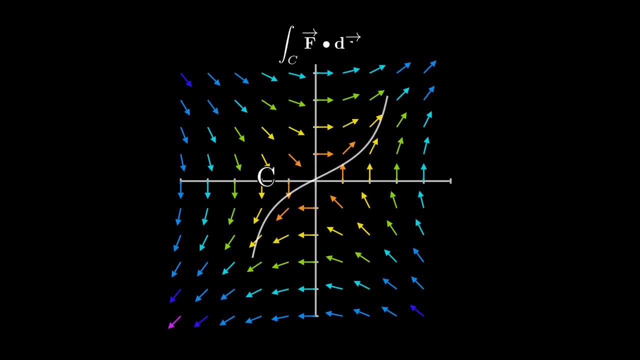 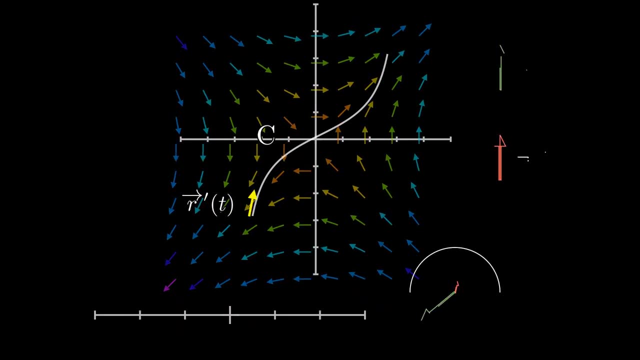 f that looks like this and is the curve c, r of t and c are the same function. To calculate the line integral of a vector field we take the dot product of plugging the curve into the vector field function with the derivative of the curve, The graph in the bottom left. 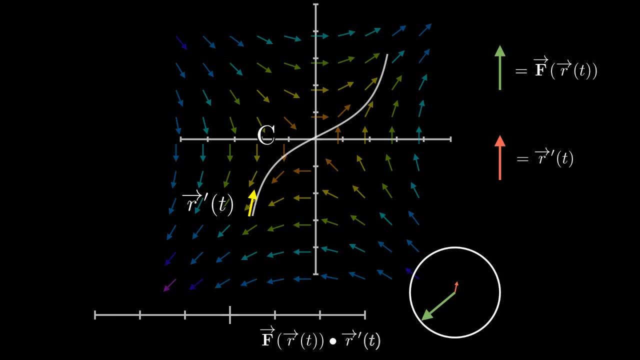 is this dot product? The circle on the bottom right shows f of r of t and r prime. This dot product gives a value that says how perpendicular two vectors are from each other. Let's play the animation out. The graph on the bottom right shows the integral. You can see how it resembles an inverse tangent. 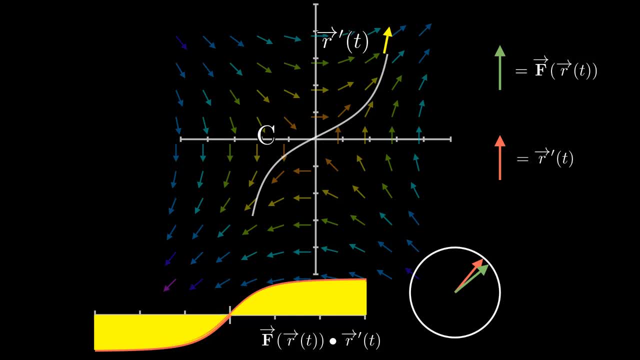 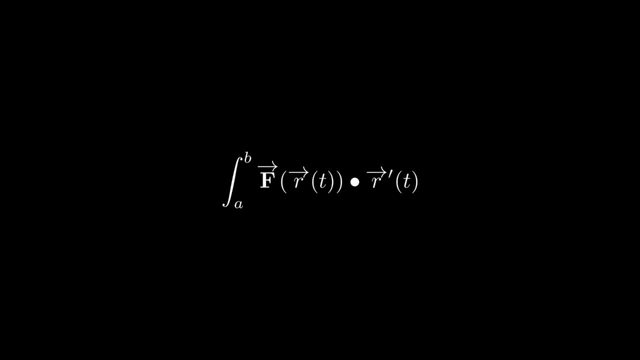 function, which this actually is. So to compute this integral, we take an integral from the vector, from a to b, of f, of r, dot, r, prime of t. There are a lot of things on the screen so you should probably pause and let it sink in. I'm gonna play the animation once more. 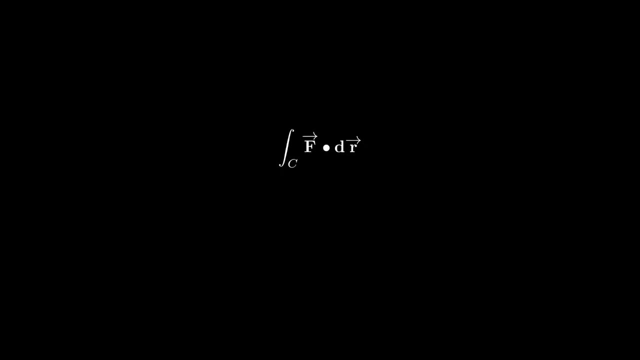 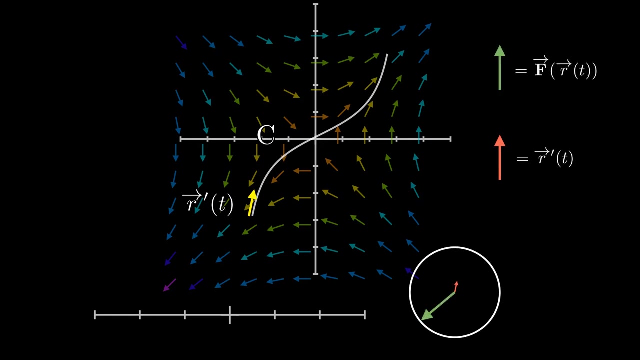 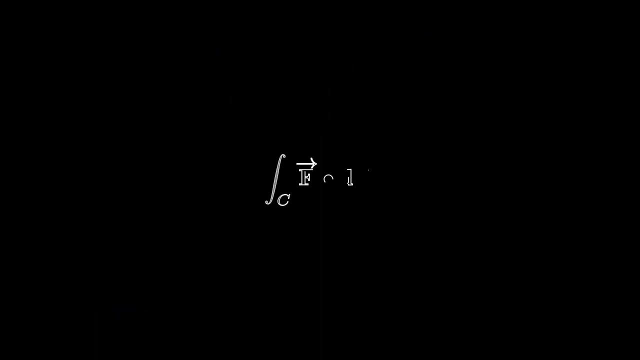 for you to see. Like last time, let's quickly go over a textbook style problem. Here's the question: Evaluate the integral of f dot dr, where f of x comma y is y squared, i hat plus three, x minus six, y, j hat And c is the line segment from three comma seven to zero comma twelve.